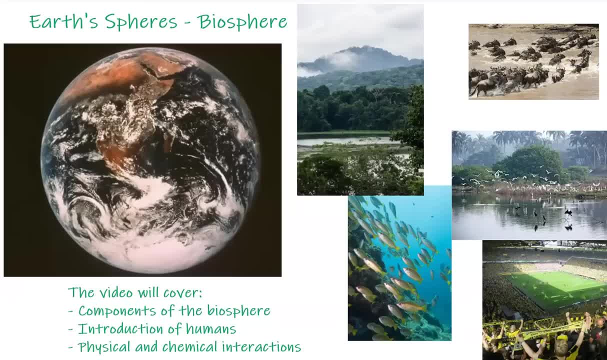 The introduction of humans, anthropogenic effects and humans as a part of the Biosphere, part of the animal kingdom, And then looking at the physical and chemical interactions that go along within these different types and different sections of the Biosphere and how they all work together and some examples. 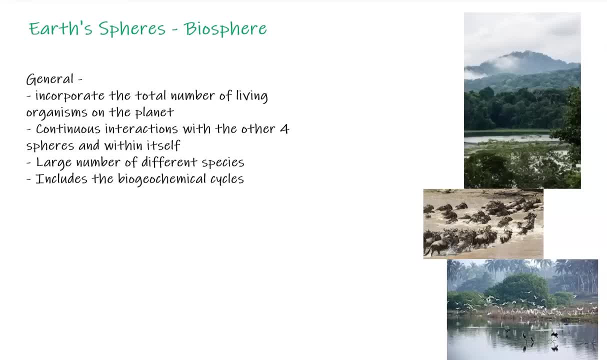 So the Biosphere in general. looking at the total number of living organisms on the planet, so the whole system is added up in one big number, all the different species. looking at the constant and continuous interactions with the other four spheres, with the Hydrosphere, the Atmosphere, the Cryosphere and the Geosphere. 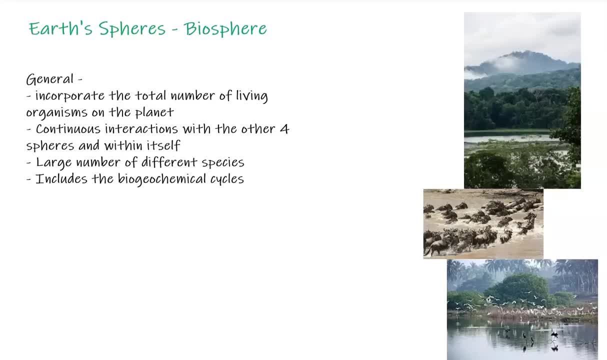 Those constant interactions are going on all across the planet with all the different species And also within the Biosphere itself, how these animals interact with each other. So, looking at the division of ecology and symbiotic relationships and all those different other topics and subjects that come into ecology, and looking at the natural world, 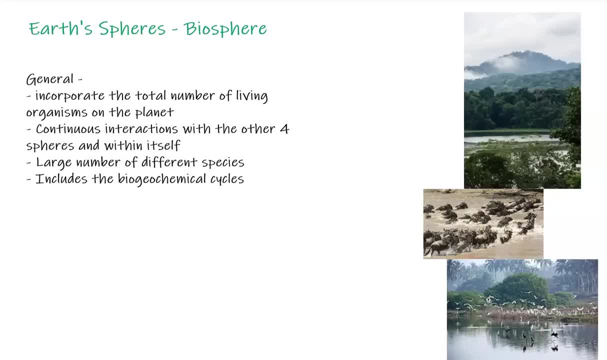 Looking at the huge amount of species that this planet holds currently in the millions of different species, But they estimate. various articles estimate between 8 and 15 million species have been on this planet since the start of oxygenation event in the Atmosphere. 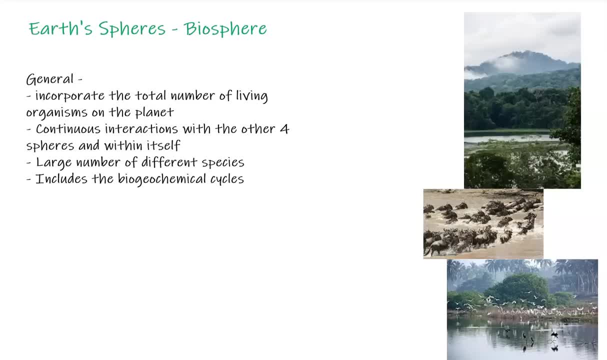 the start of the single cell bacteria and organisms that come from the ocean and develop from there. So 8 to 15 million different species- One of them is Homo sapiens- And then, basically, that being said, over 99% of all those species are now extinct. 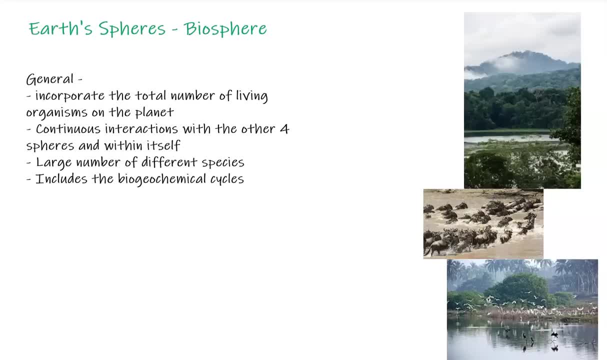 And we're just left with the current one. It's the only one that has been on the planet yet. So are there more species that we're still learning or we are seeing, or one percent that we are still know about, or there's more species that we are still finding out and discovering around the world with each year. 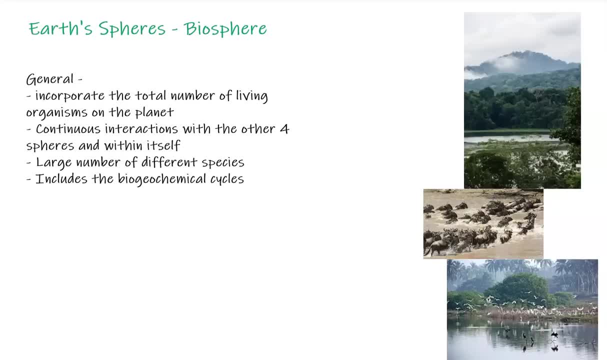 We're looking at the biogeochemical cycles as well, looking at all of the cycles involved, with both the carbon cycle, the phosphorus, nitrogen, potassium cycles, the most popular common ones. Also, you can include the water cycle as well. 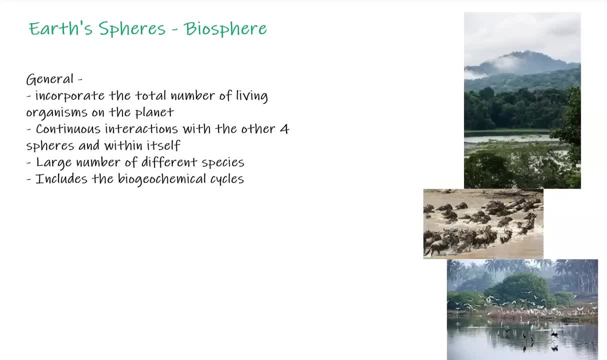 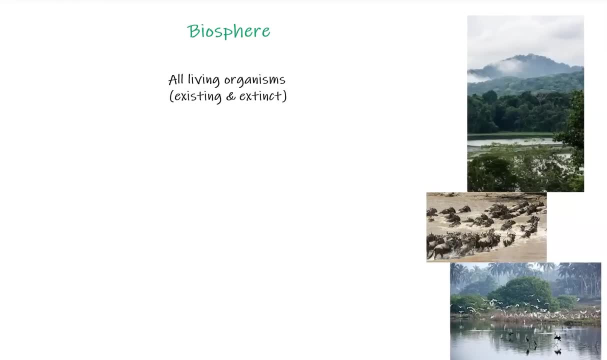 And maybe as well the rock cycle, if you will. There's much more to be discovered in the future cycle, because it also involves different elements within the minerals that create the rocks, then then go through the cycle, so the biosphere. let's start at the beginning. so again, definition is all. 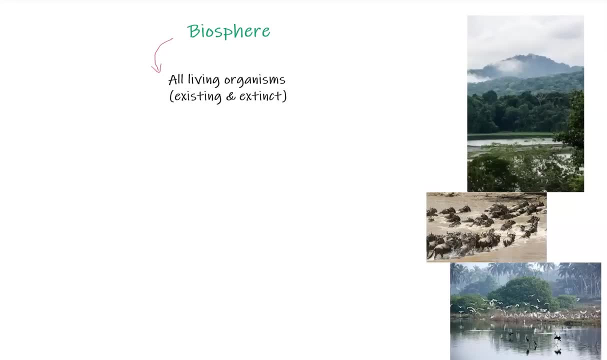 living organisms, all the currently existing organisms and the ones that are extinct from the past, and we can also discuss this as biota as well. so to get the biosphere to start to initiate the organisms and life, we need energy. so the energy principally comes from the sun. 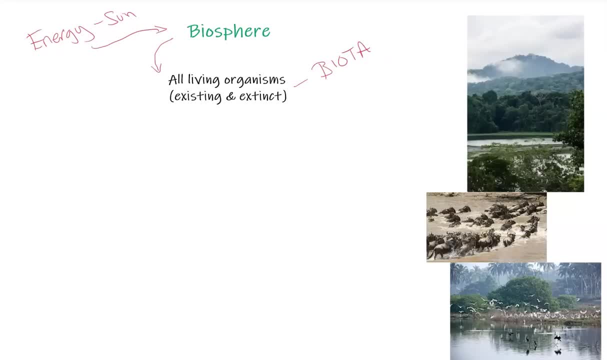 and then the transfer of energy through various other means and physical processes are going to go through the biosphere and promote life and also the promotion of the cycling of energy and elements and matter. so through the biosphere, through those biogeochemical cycles discussed a minute ago, so we can characterize. 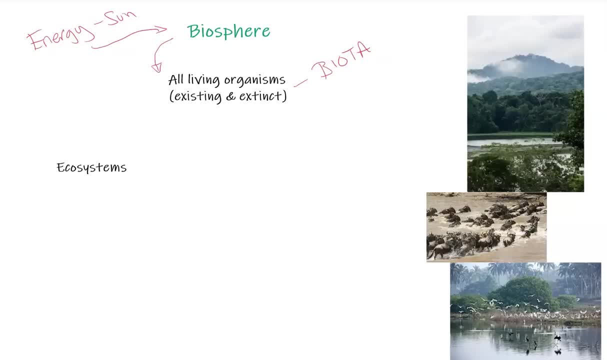 and put in place areas of the planet that have certain set landscapes, terrains, vegetation and species, and these are called ecosystems. so there are various ecosystems all across the planet and we can, you know, characterize them in certain ways, based on their climate, based on their terrain, vegetation. 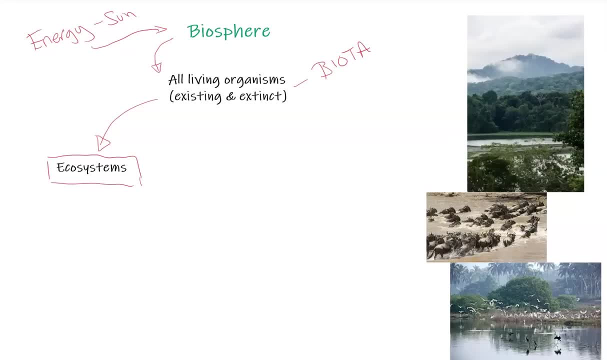 and the species diversity or range of species that live in that ecosystem and that changes across the world, across the continent, based on the various factors of climate and terrain and a bit of food and also habitats. so we can look into that. we can break this down to a lot of. 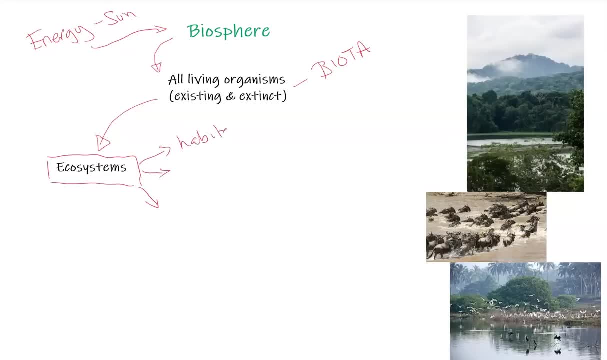 different things. so we can do the habitat, we can do the, the food source, we can do the species. we can do the uh the food source, we can do the species, we can do the uh topography and terrain interactions which would promote a certain ecosystem. so we 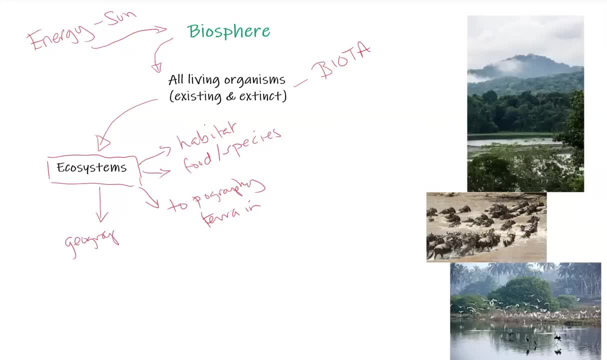 can do location, so a little bit of geography can also come into this, where their located in certain places in the world. so next we can add in biomes. now biomes differ a little bit from ecosystems. ecosystems are the flora and fauna plus the physical environment. so you can bring 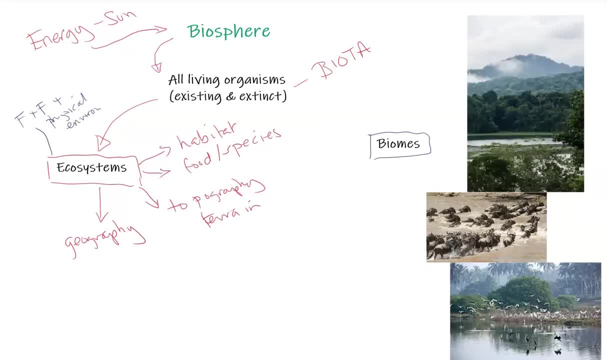 in a lot of the physical attributes of an area and that would dictate the diversity or the extent of flora and fauna growing in that area or existed in an area. but biomes is just purely flora and fauna. now, flora and fauna means animals and plants. okay, flora is the plants of vegetation, fauna is the. 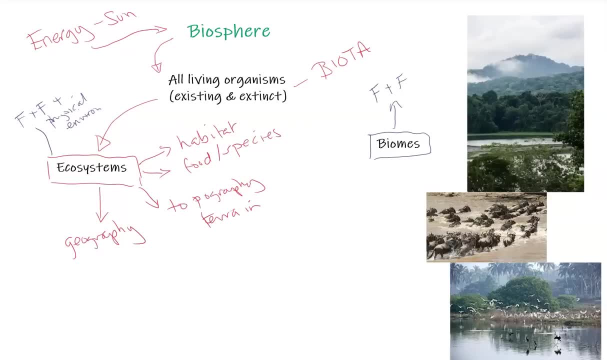 different kind of species of animal that inhabit that area. so biomes can be closely linked to ecosystems. but also they are one section of the biosphere where these living organisms reside or have their habitats. so we can also have biomes, we can have location. certain biomes occur in certain places in the 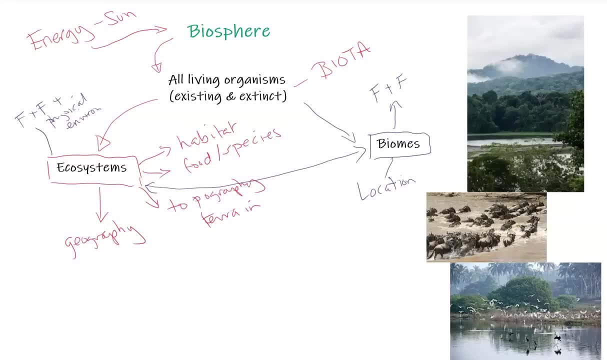 world because of the climate and the terrain. I can also discuss the types. now the biomes are different from each other. they are different from each other. they are different from each other. so biomes are dictated by pretty much temperature and rainfall or precipitation. so temp and precip are the kind of defined. 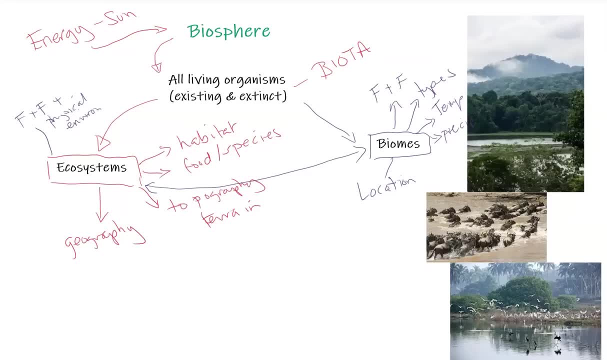 factors that would govern a biomes development and where they are, and they can change over time. so, over over the history of the earth, over geologic history, you've had areas of the world which have changed drastically in terms of their ecosystems and biomes. the Sahara Desert, for example, was lush and green only between seven to ten. 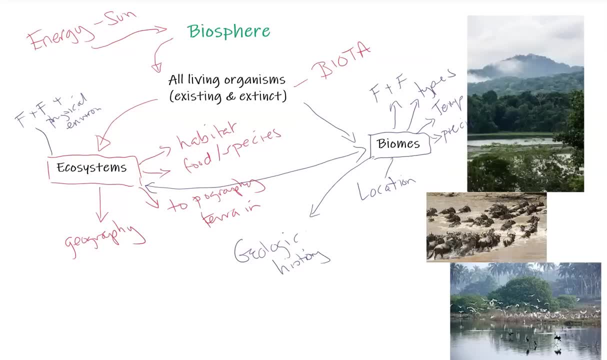 thousand years ago and was a was a myriad of different river and fluvial systems over the whole Sahara Desert in North Africa and now it's basically a very large desert- mostly sand, but very large desert. so it's changed drastically from nice grasslands and different types of large animals like you get in Serengeti. 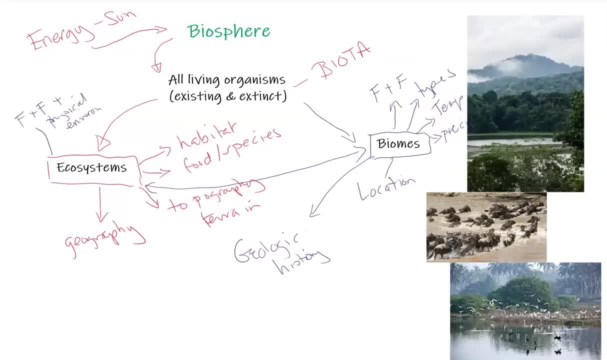 present dayceğim and Mariö, fresh ice and green rice, desolate desert, pretty much So. the next one is biomass. Biomass is the total weight of a species in a certain area. Now, the more the increased amount of species in a given area you're going. 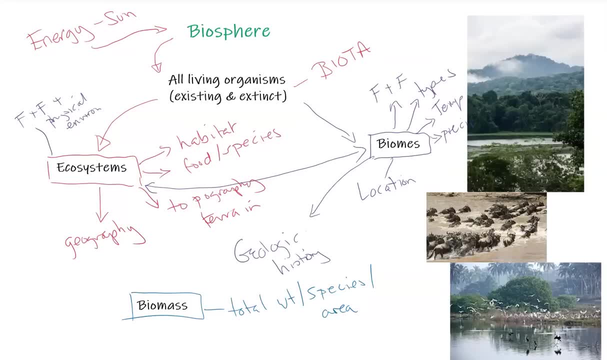 to increase the biomass. And the biomass is an indication of the health of the environment, of the ecosystem or of the biome. And the health is a result of the conditions. And the conditions are set by both the climate, both the location, the geographic and physical. 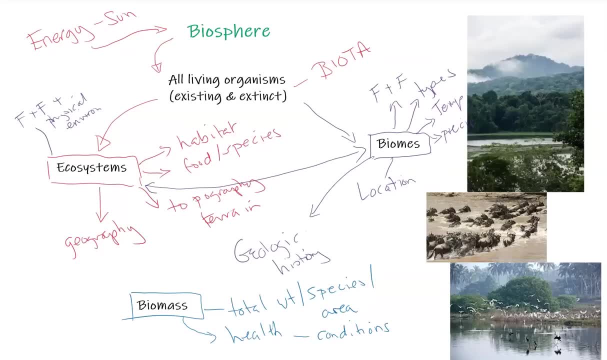 environment And those conditions would dictate the health And that will be shown in the biomass, with the large species diversity, the large amount of species in a certain area and the sustained development And the biome is the source of that biome or ecosystem over a long period of time, For example. 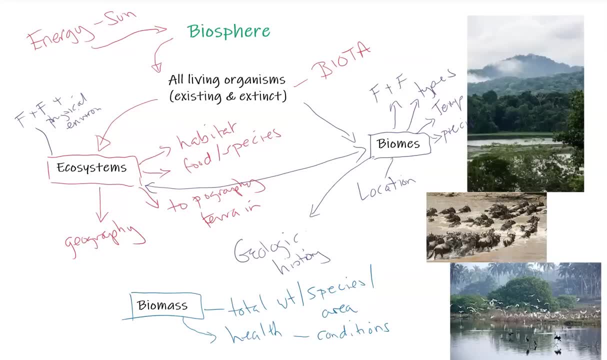 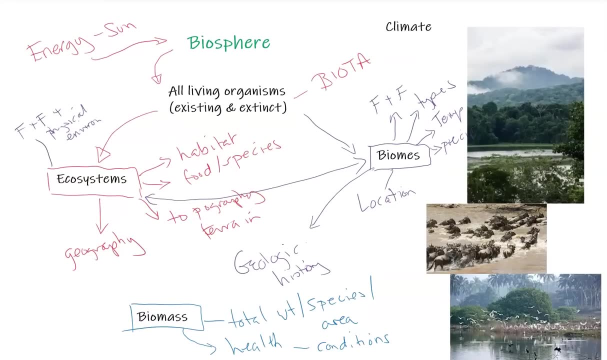 the Amazon rainforest, Lush productive, high biomass, high productivity and a very large range of both flora and fauna. The next thing to add into the biosphere, which really is like a secondary or even an initial catalyst for the whole biosphere, is the climate. Now, Earth's climate in general is conducive to. 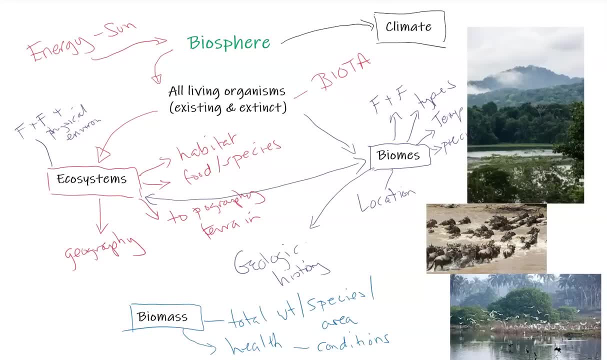 allowing life to prosper, with the addition of water and the right gases in the atmosphere and the right distance from the earth, The right system of astronomical processes that make up the ability to have life on this planet, as opposed to life on Venus or life on Mars Or maybe another. 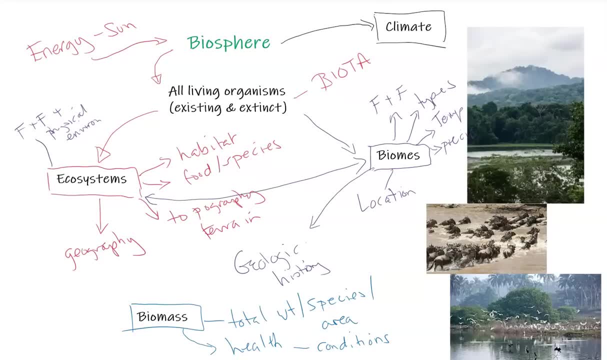 planet further away, But we have a good, sustaining life climate now. It does change and fluctuate in different locations and, according to NASA, in most areas of the climate that our planet's planet has Just bypolizing the climate it makes up a greater chance of having life. So a lot of the 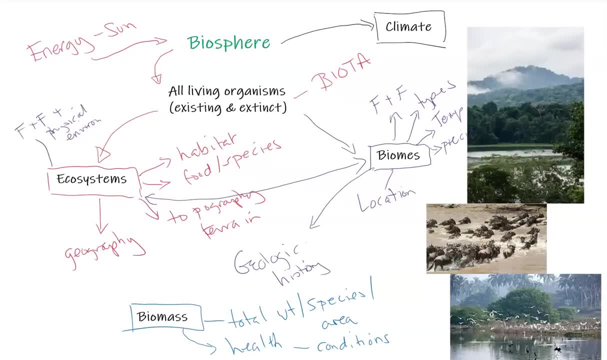 latitude according to the solar concentration. but climate is a huge factor which dictates the biosphere. Now the biosphere can also dictate the climate. Now humans are a fantastic example, Homo sapiens sapiens, of how we have dictated or fluctuated the climate in certain areas. 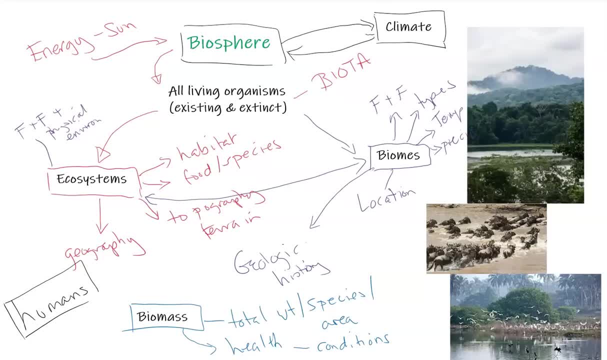 Now, I'm not talking about climate change in this video, but let's say the urban heat effect. You know a large city that is all concrete and built up like a New York City, like a Tokyo, like a Mexico City, LA. these large cities would actually change and have a microclimate. So 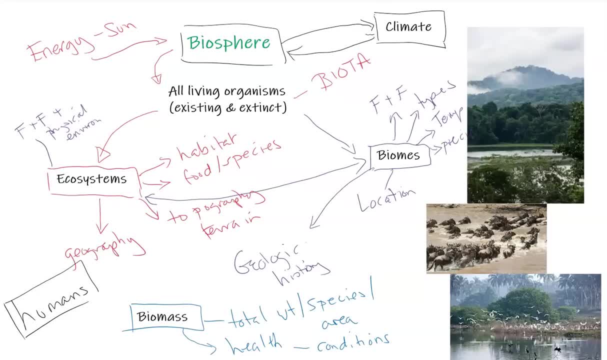 the human element, the human species, has an impact on the biosphere and on the climate of the world, And with the humans we can also add in the term the anthro scene, which is an era in geologic history that some scientists promote, and say that we're in the anthro scene as 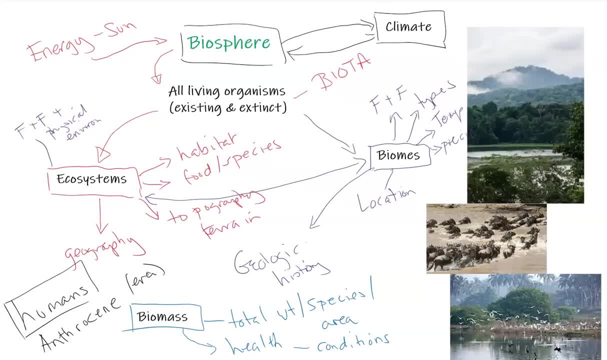 a new part of history, of geologic history, and also in terms of spheres. Oh wait, There we go, Anthrosphere being the sphere of mankind, the sphere of Homo sapiens. So an additional sixth sphere to appreciate and combine all the different variables that humans 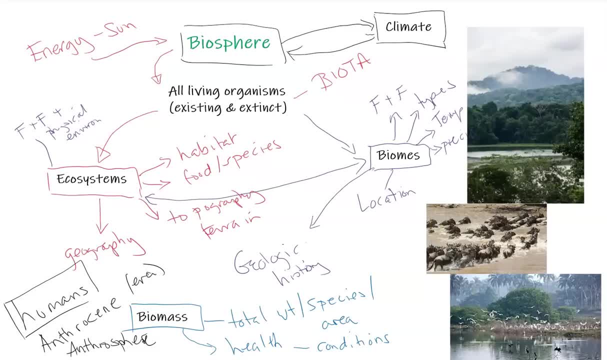 bring to planet Earth. So, in addition to the cryosphere, the atmosphere, the hydrosphere, the geosphere and the biosphere, would be the anthrosphere. So, in addition to the cryosphere, the atmosphere, the hydrosphere, the geosphere and the biosphere, 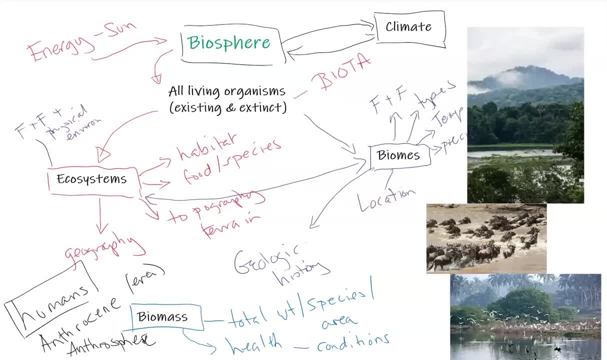 which is just humans and the interactions that we have on this planet, And unfortunately maybe a bit too large of interactions. And the last main component of the biosphere is going to be the soil and lithosphere. So between 10 to 30 percent of all living organisms reside or have the habitat or are 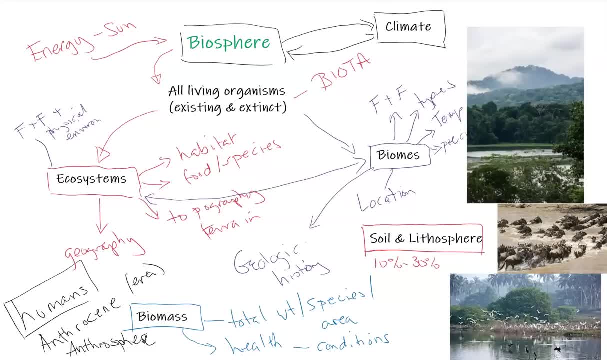 underground. So it could be just the initial few feet, or it could be deep underground in the lithosphere, in various areas- Yeah, no, 천caесcares- or in between the rocks and bedrock. But the soil is that perfect interface of the biosphere, the geosphere, atmosphere, hydrosphere. 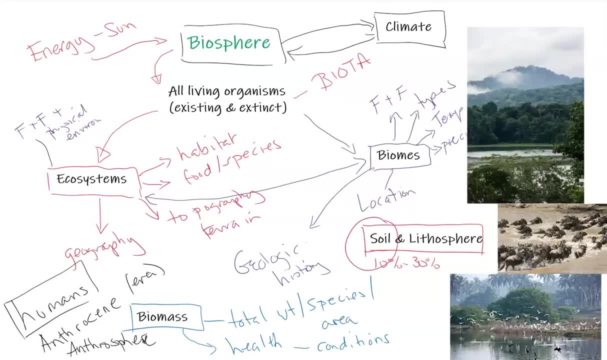 and all of the biochemical cycles. They all go through the soil. So it's very important to appreciate the role of soil in the biosphere, not just for habitats and where animals live, but also the interactions with the other spheres and the lithosphere. 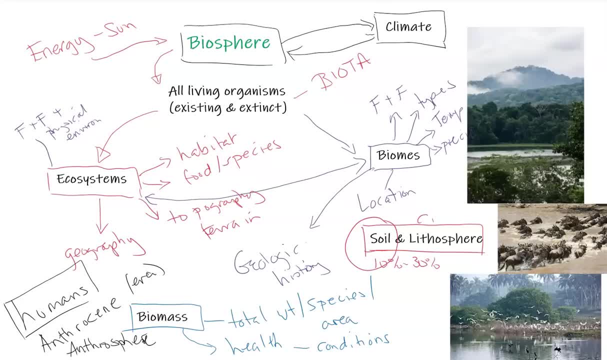 That's the crust lithosphere combined which forms the upper mantle, is going to be again that the area of study where a lot of the animals reside not just on the surface but the subsurface realm or regions as well. so I hope this explained the biosphere and broke it down into its different components. again you can go.